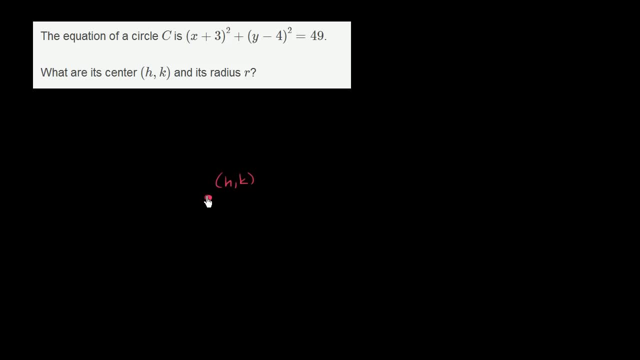 The circle is a set of all points that are equidistant from that point. So let's take the set of all points that are, say, r away from hk. So let's say that this distance right over here, this distance right over here, is r. 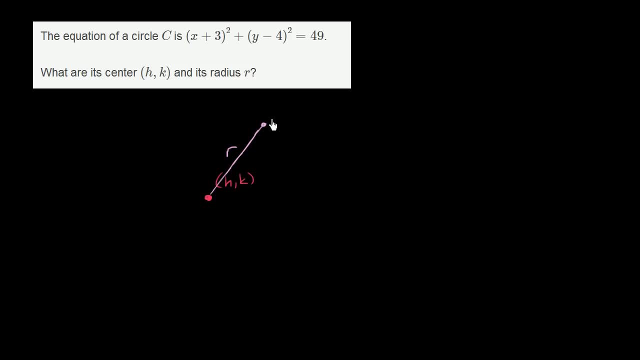 And so we want all the set of points that are exactly r away, So all the points x, comma, y that are exactly r away, And so you could imagine, you could rotate around, and all of these points are going to be exactly r away, And I'm going to try my best to draw at least. 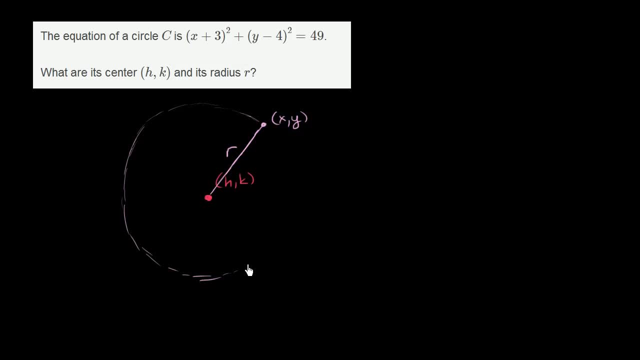 a somewhat perfect looking circle. I won't be able to do a perfect job of it, But you get a sense. All of these are exactly r away. at least if I were to draw it properly, They are r away. So how do we find an equation in terms? 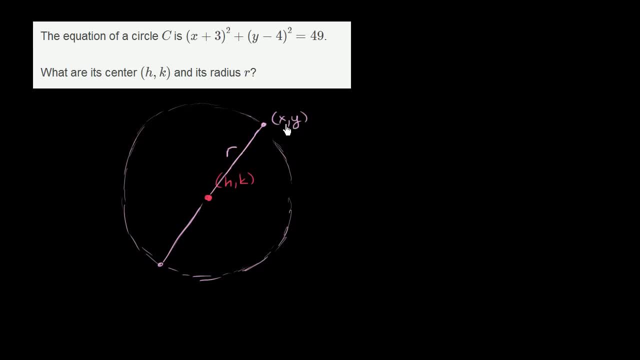 of r and hk and x and y. that describes all these points Well. we know how to find the distance between two points on a coordinate plane, And in fact it comes straight out of the Pythagorean theorem. If we were to draw a vertical line right over here. 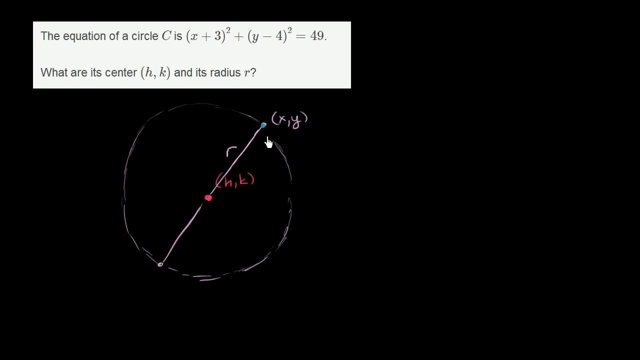 that, essentially, is the change in the vertical axis between these two points. up here we're at y, Here we're k. So this distance is going to be y. Here we're y minus k. We can do the exact same thing on the horizontal axis. 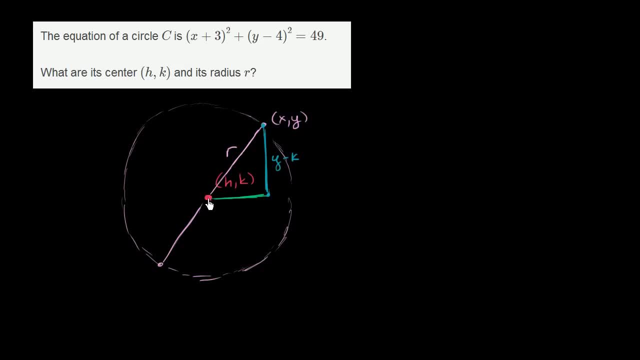 This x-coordinate is x, while this x-coordinate is h, So this is going to be x minus h. is this distance? And this is a right triangle, because by definition we're saying, hey, this is a vertical, We're measuring vertical distance here. 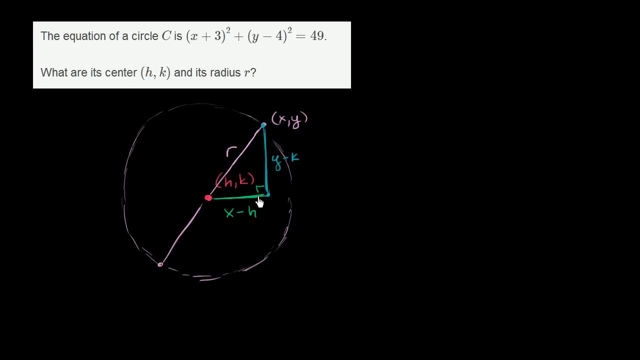 We're measuring horizontal distance here, So these two things are perpendicular, And so from the Pythagorean theorem we know that this squared plus this squared must be equal to our distance squared, And this is where the distance formula comes from. So we know that x minus h squared, plus y minus k squared.